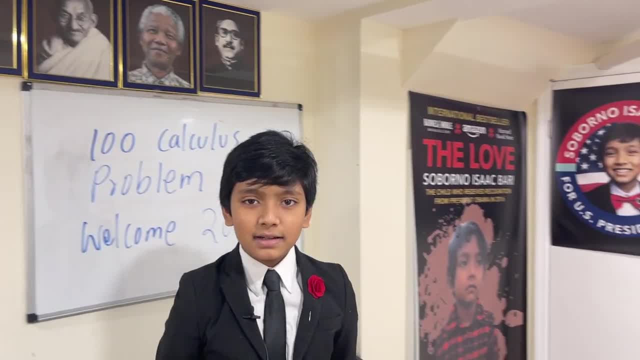 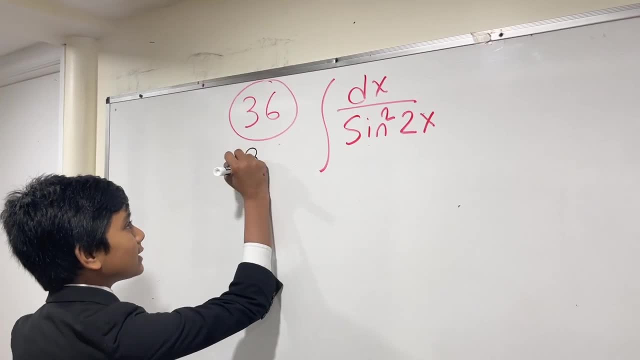 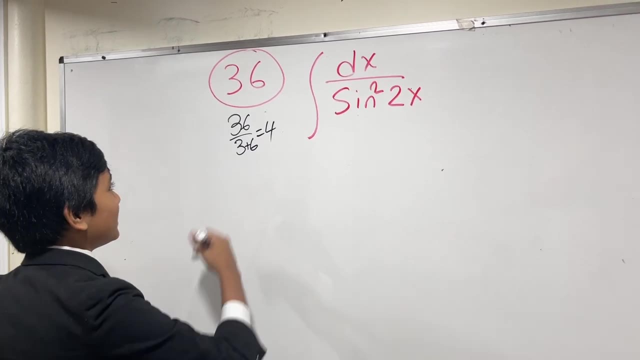 Hello everybody, my name is Sabona Isaac-Bears from BabyScienceLab, and today we are going to be doing problem number 36.. Now, 36 is actually a hard-shaddened number, because 36 over 3 plus 6 is 4.. Wow, Outstanding. 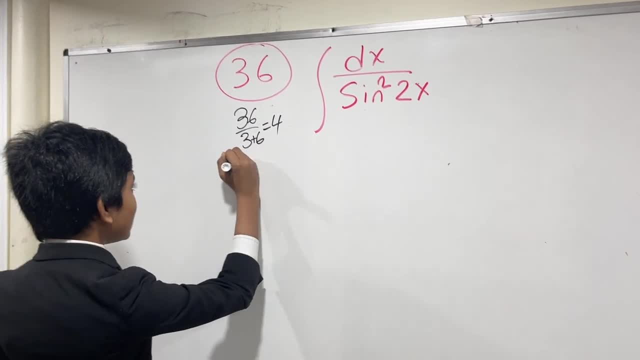 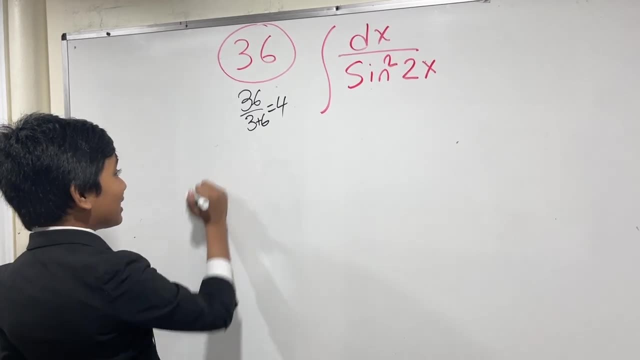 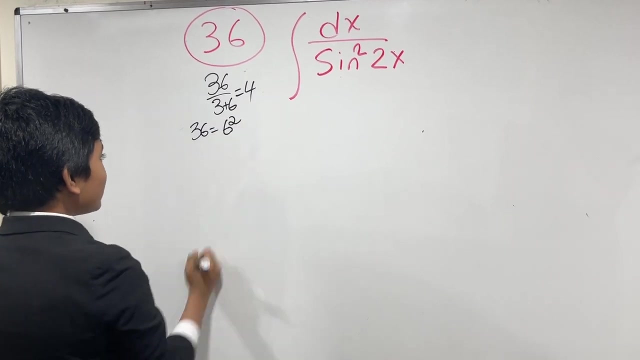 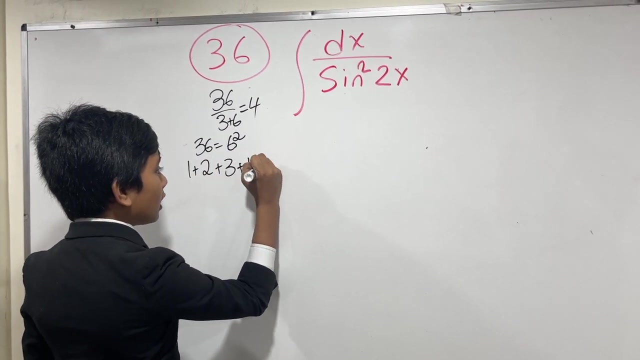 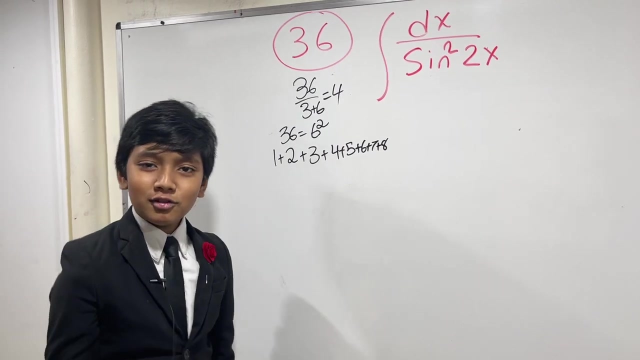 So also the sum of 36 is a tri-square number. Why, Well, that's because tri-square? That's because 36 is equal to 6 squared. and 36 is also equal to, if I remember correctly, 1 plus 2 plus 3 plus 4 plus 5 plus 6 plus 7 plus 8 plus 0 plus 0 plus 0.. Cool right. 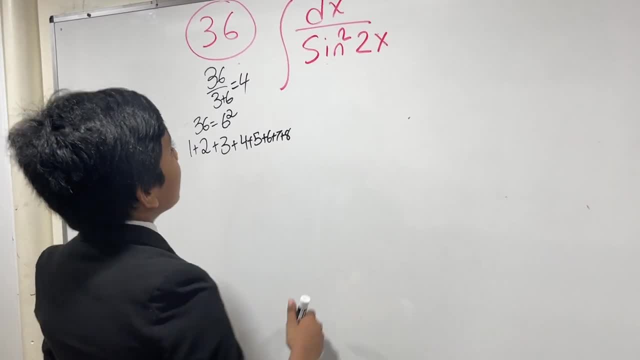 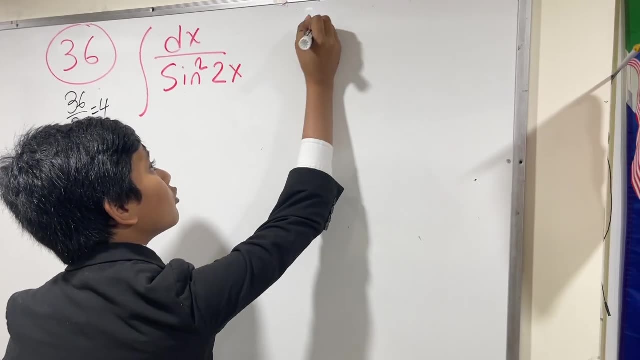 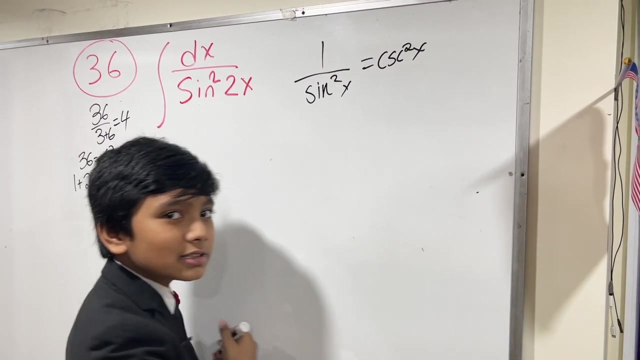 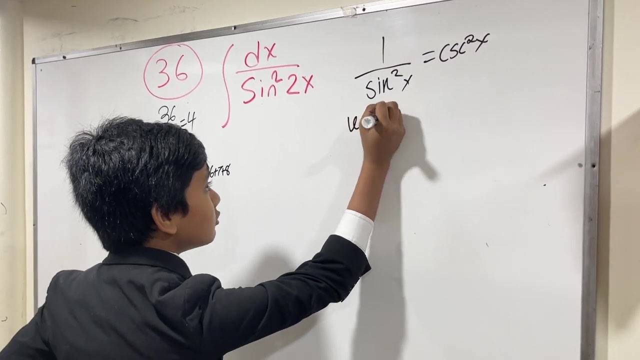 Okay, so dx over sine squared 2x. Well, the thing-o-hero is that oh 1 over sine squared x can simply be written as cosecant squared x. So what do we do here? Well, I guess we use up: u is 2x, dx is du over 2.. 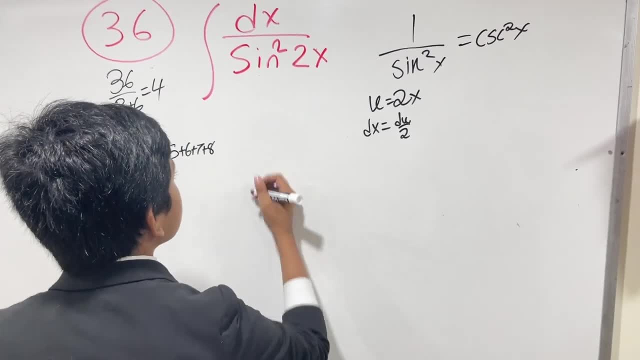 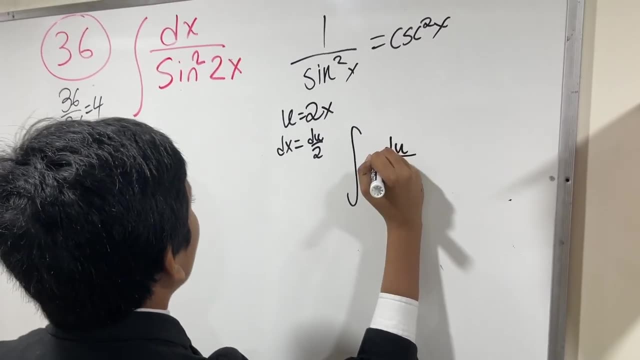 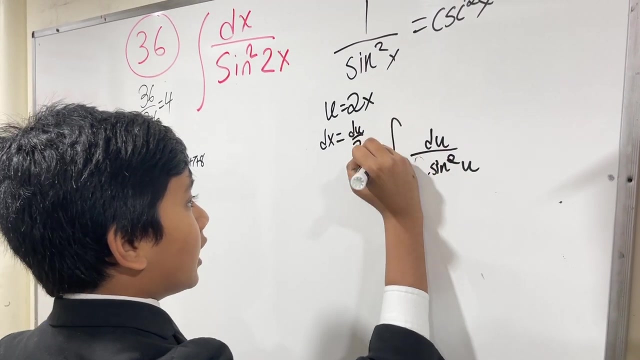 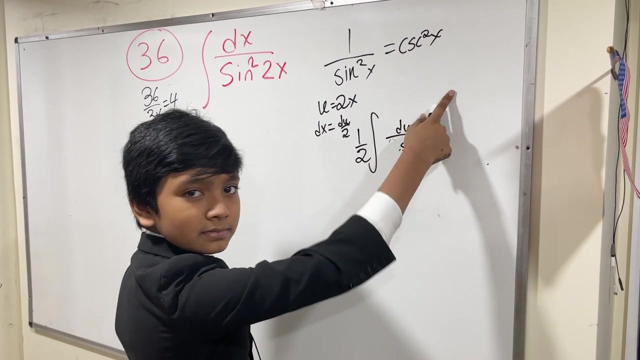 Watch problem 5 if you don't understand. So we get the integral of du over 2 sine squared u, And I guess we can just bring that 2 outside, All right-o. So now, uh yeah, 1 half cosecant squared u du. 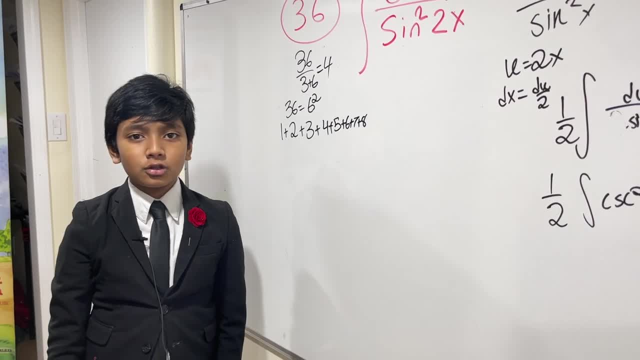 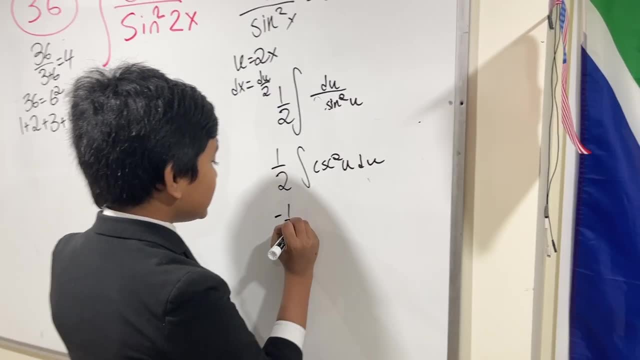 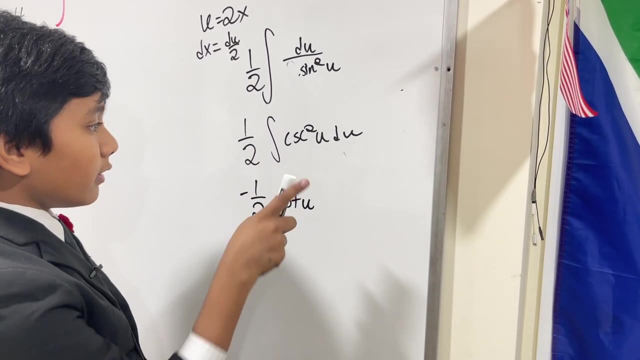 And you may or may not have noticed that this looks similar to the derivative of tan x, which is secant squared x. Well, you've got that one right, Because this is simply just minus 1 half cotan u. But uh, because the derivative of negative cotan u is actually cosecant squared u. 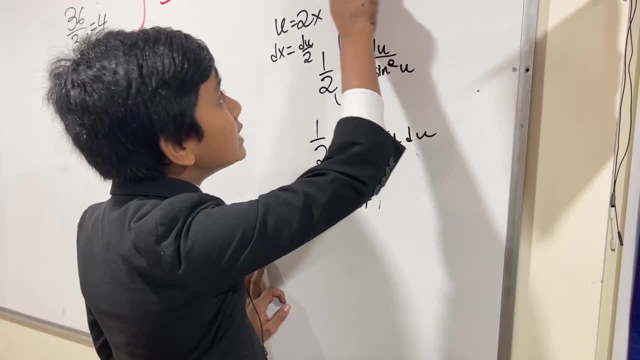 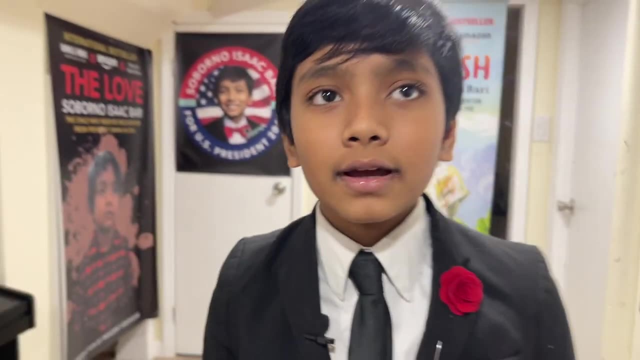 Pretty cool, right? And now we unsub u, which is: where was it? 2x, That's the answer Plus c. Thank you everybody for watching. We'll see you in the next one. Hmm, Suborno Isaac Bari.